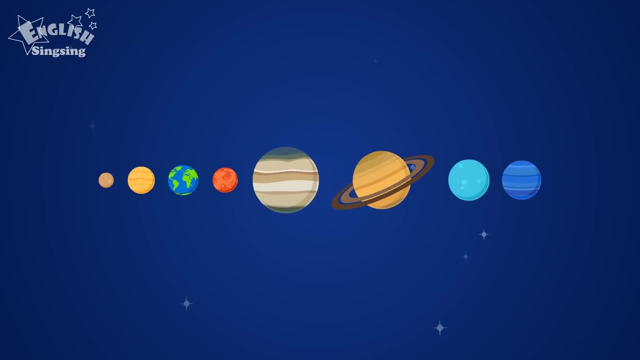 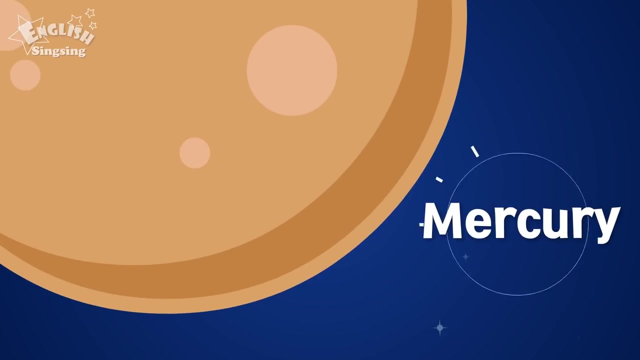 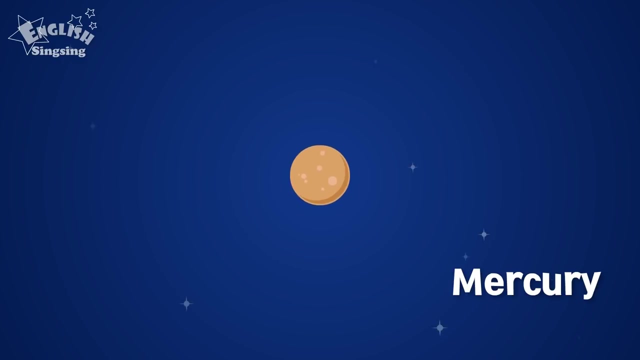 Mercury, Venus, Earth, Mars, Jupiter, Saturn, Uranus, Neptune and Sun. Mercury- Mercury is the closest planet to the sun, Venus- Venus is the brightest planet in the sky. Earth- Earth is our planet. Mars- Mars is a red planet. 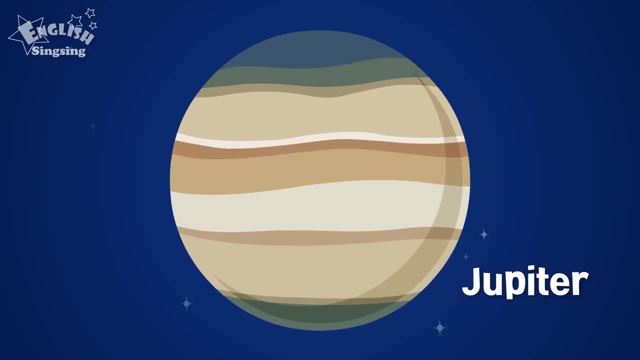 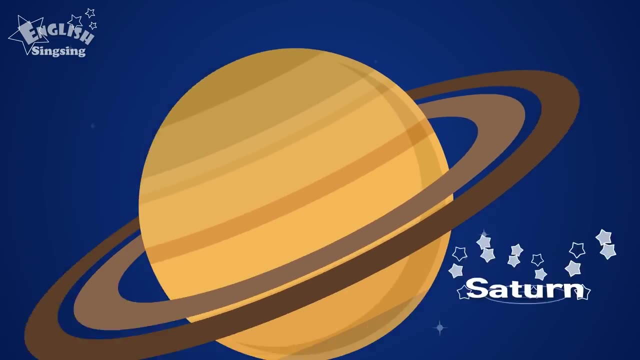 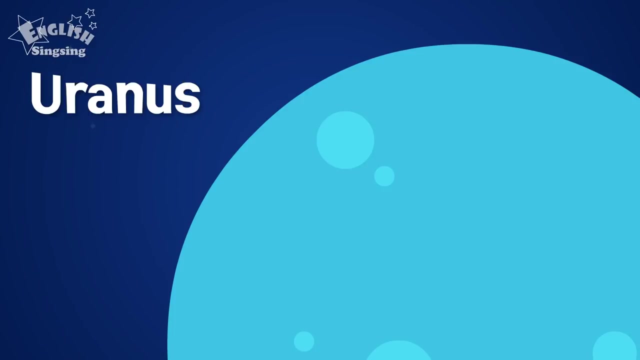 Jupiter: Jupiter is the largest planet. Saturn: Jupiter is the largest planet in the sky. Saturn: Saturn is the planet with the rings. Saturn is the planet with the rings. Uranus: Uranus is very cold and cloudy. Uranus is very cold and cloudy. 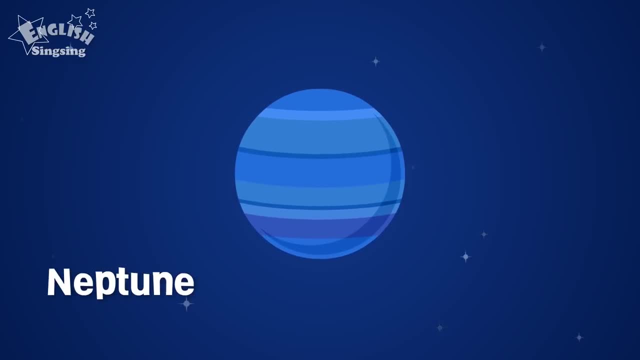 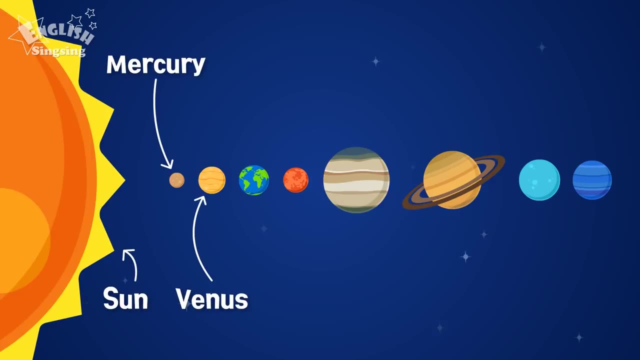 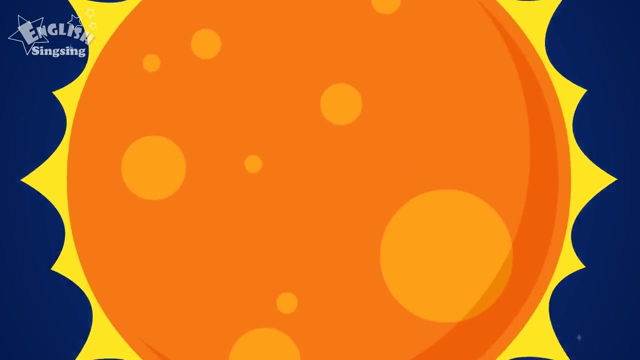 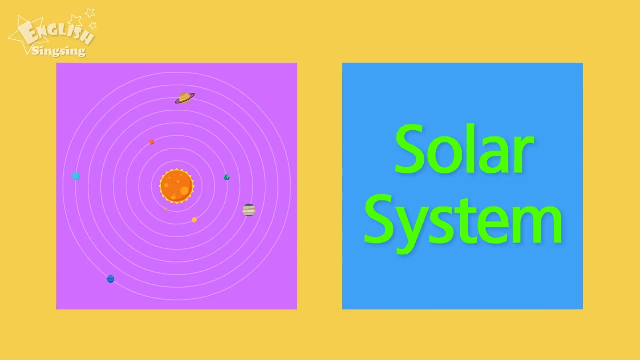 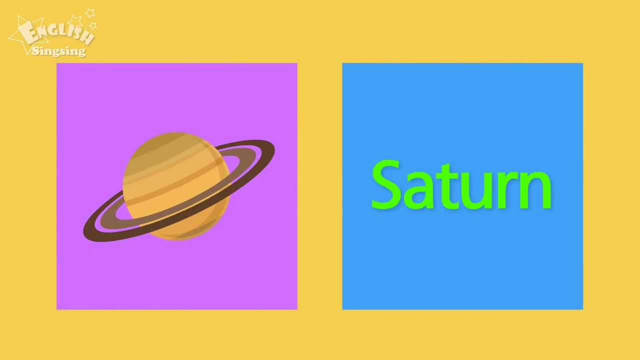 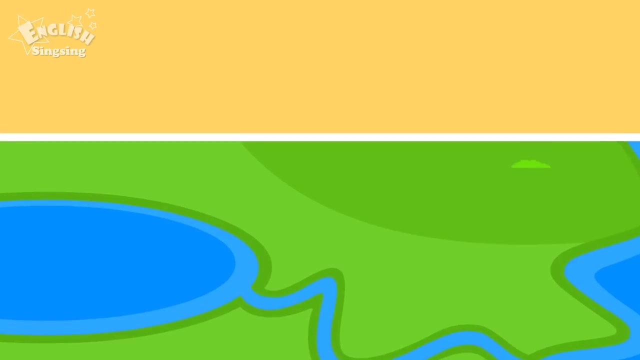 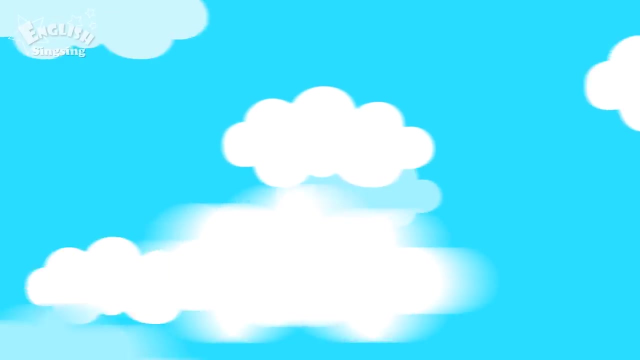 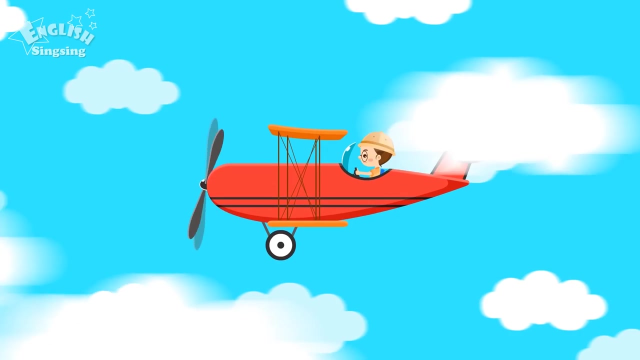 Neptune. Neptune is made of gas. Sun, Sun, Mercury, Venus, Earth, Mars, Jupiter, Saturn, Uranus, Neptune. This is our solar system Review. Solar System: Sun, Mercury, Venus, Earth, Mars, Jupiter, Saturn, Uranus, Neptune, Geography Sky. The sky is so high. 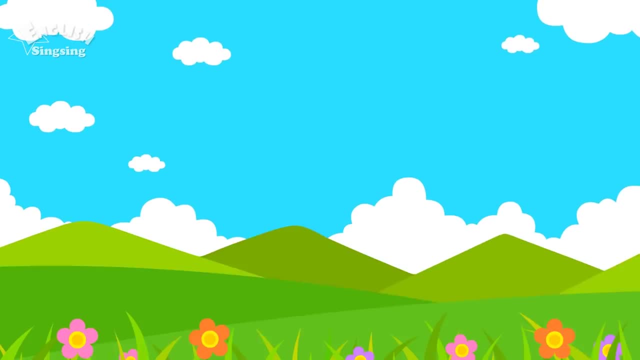 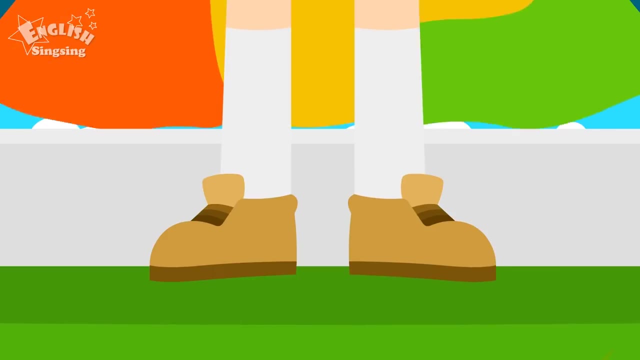 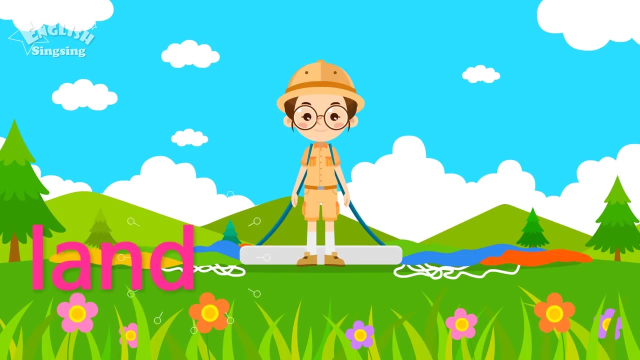 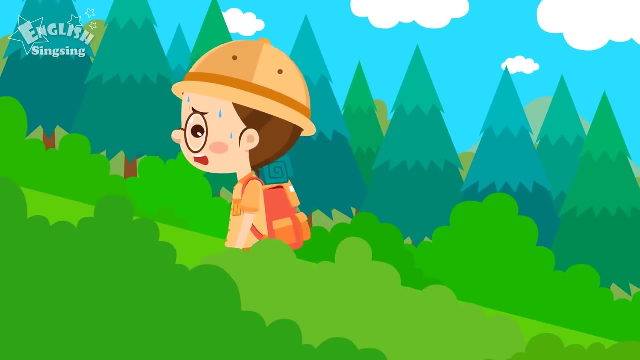 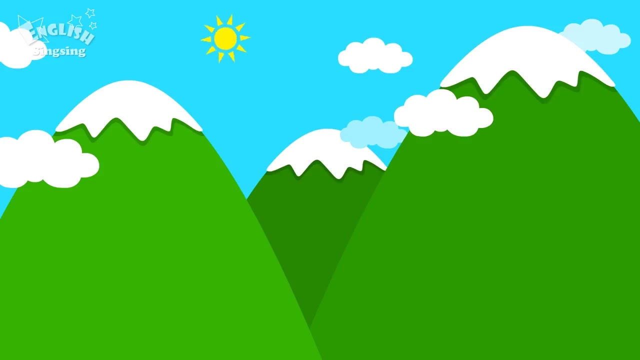 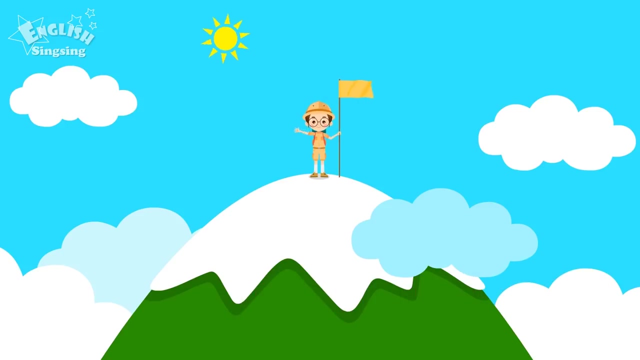 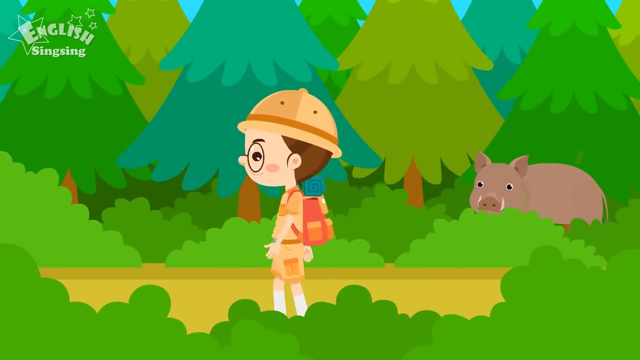 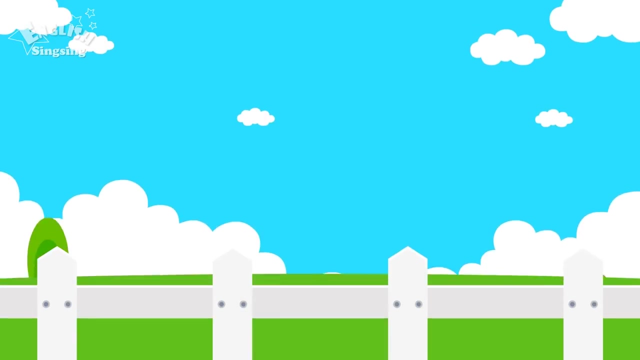 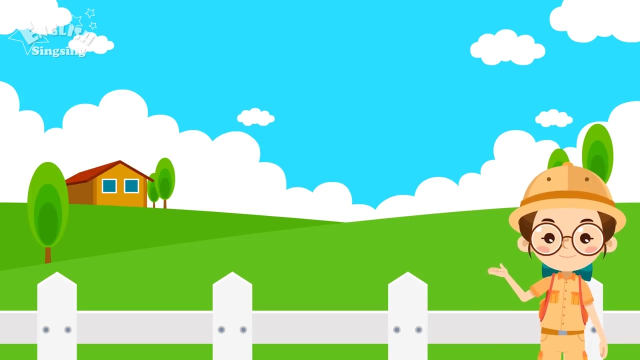 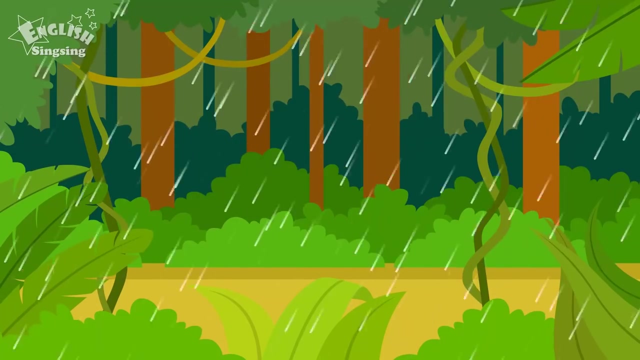 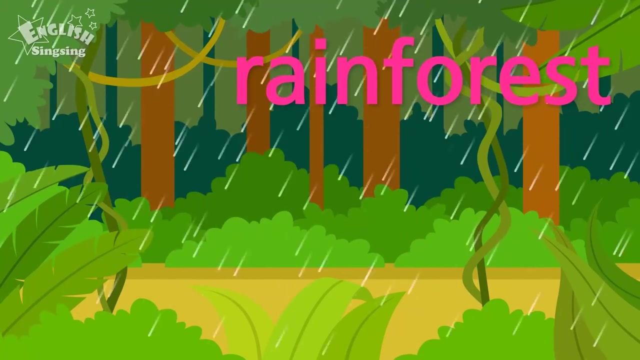 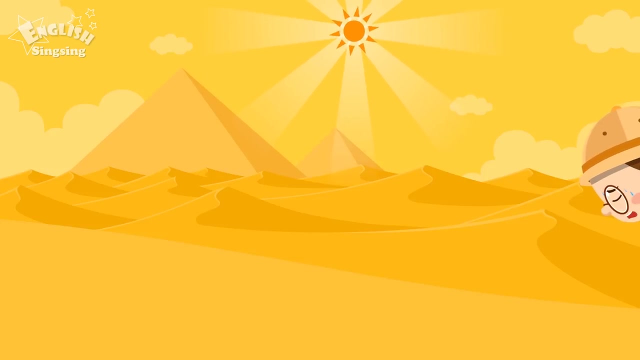 Sky, Land, Land. We are standing on the land, Land, Mountain. The mountain shoots up, Mountain Forest. Many animals live in a forest, Forest, Field. There are wide green fields, Field, Field, Rainforest- A rainforest has lots of rain, Rainforest, Desert- A desert is a very hot and dry place. 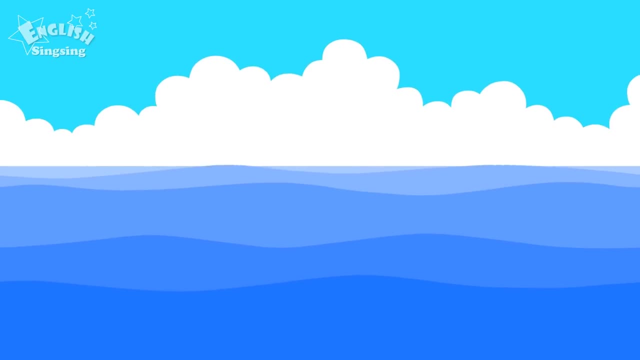 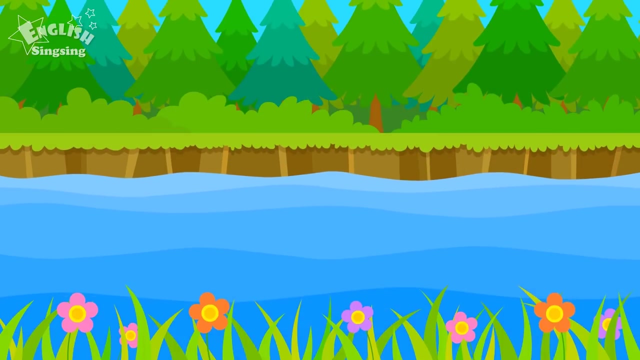 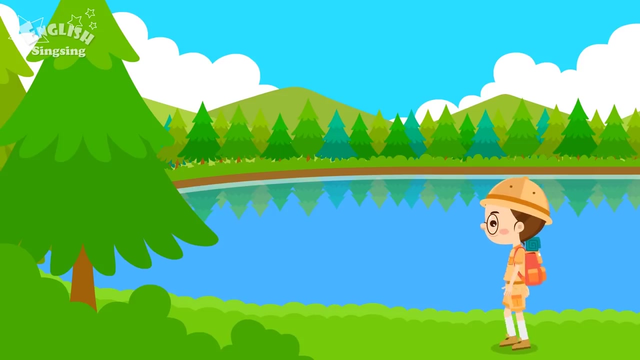 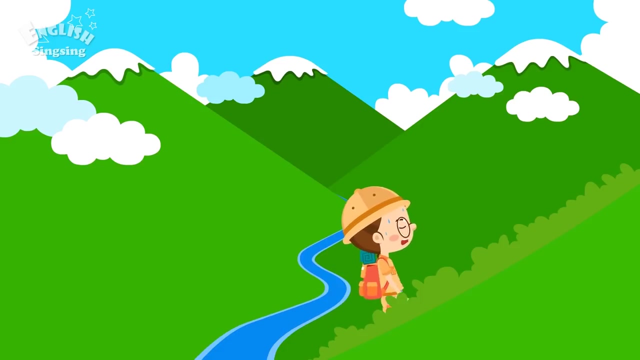 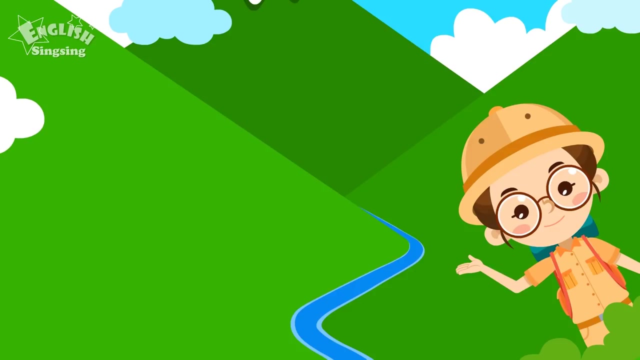 Desert Sea. The sea is very deep, and blue Sea Island, An island, is surrounded by the sea Island River River. A river flows into the sea River Lake, A lake is as smooth as a mirror. Lake Valley, A valley, is a lowland between two mountains. 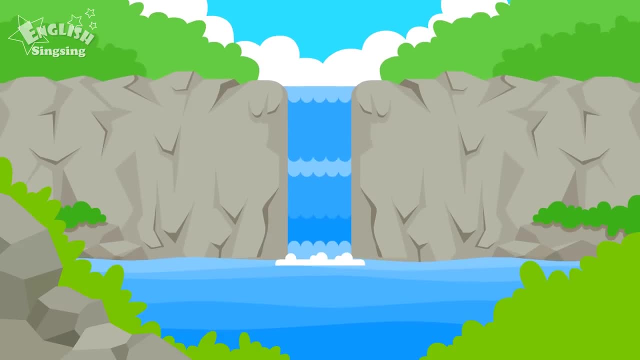 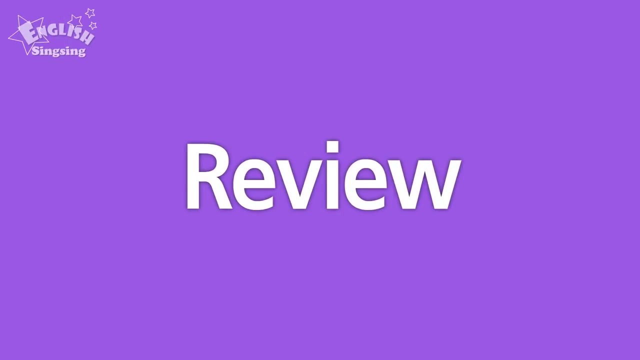 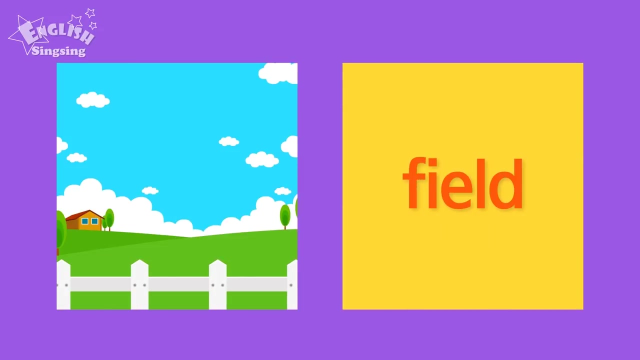 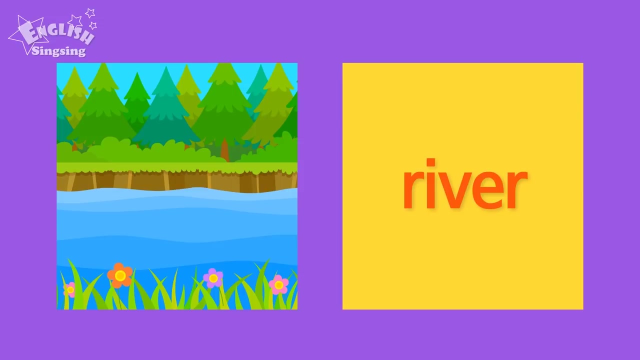 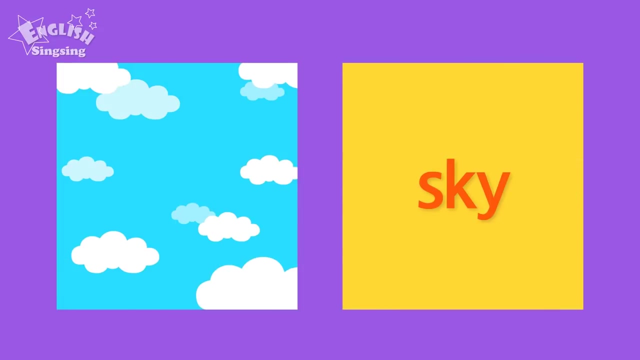 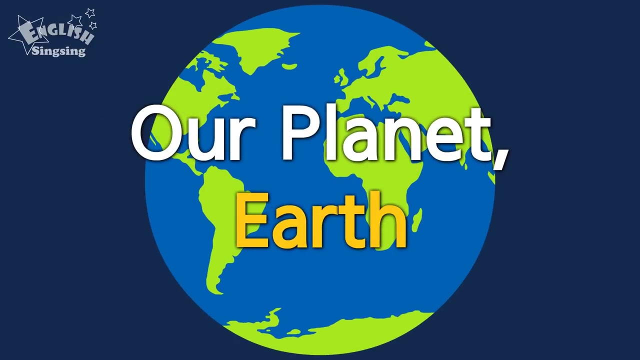 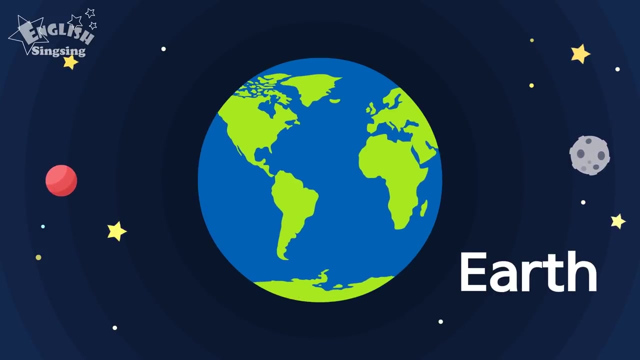 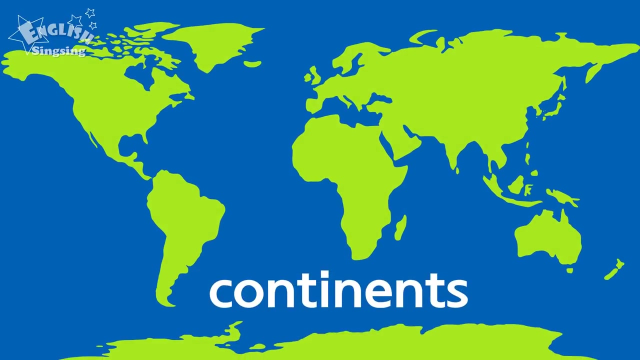 Valley Waterfall. A waterfall falls from a cliff Waterfall. Desert Field, Forest, Island, Lake, Land, Mountain, Rainforest, River, Sea, Sky Valley Waterfall. Our Planet Earth, Earth, This is the blue planet Earth. This is the planet Earth we live in Earth Continents, There are continents on the Earth. 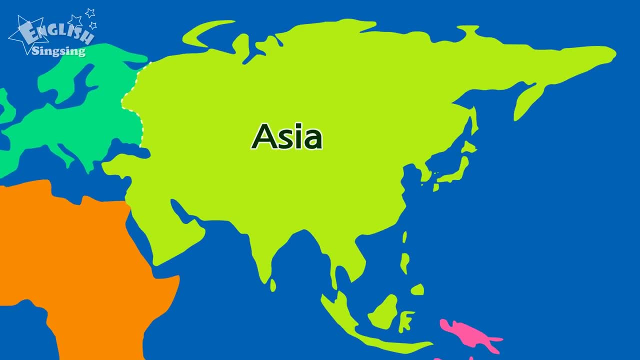 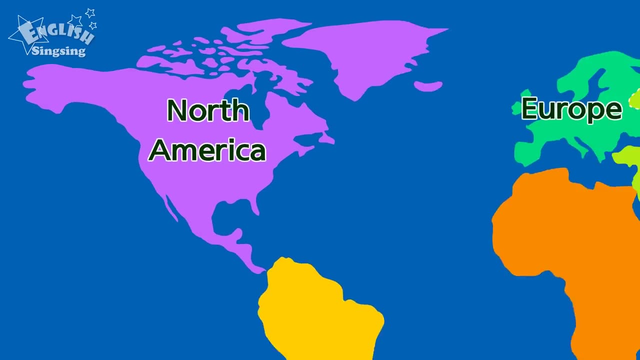 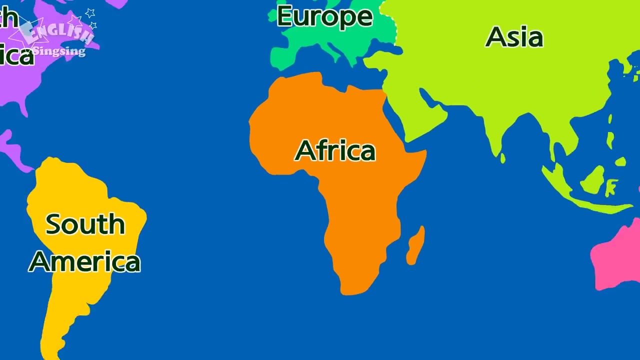 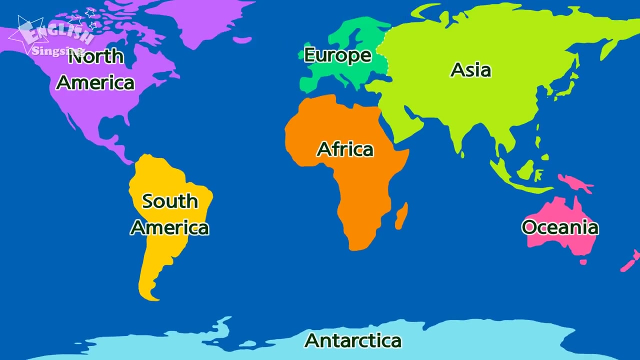 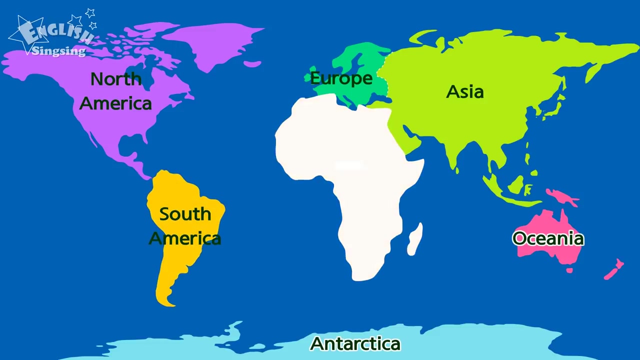 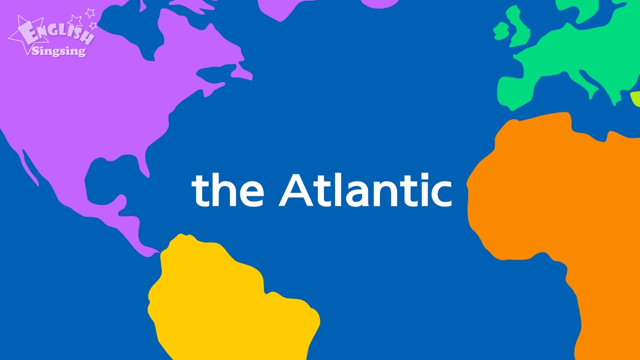 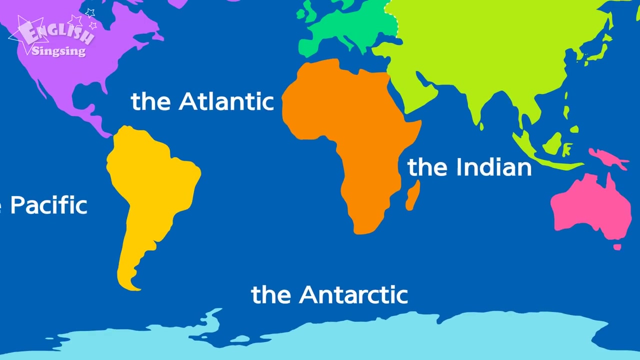 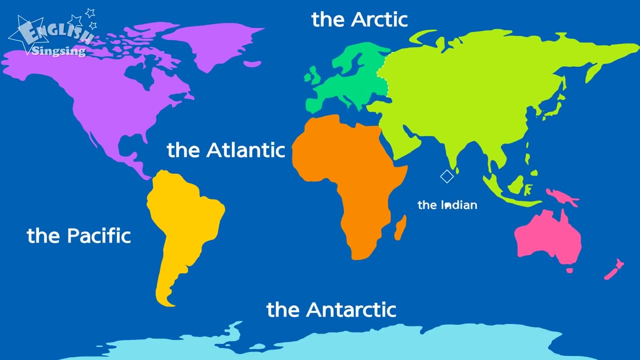 Continents: Asia, Europe, North America, South America, Africa, Africa, Oceania, Oceania. Antarctica. Antarctica- Asia, Europe, North America, South America, Africa, Oceania and Antarctica. Oceania Oceans. There are oceans on the Earth Oceans: the Pacific, the Atlantic, the Indian, the Antarctic, the Arctic, the Pacific, the Atlantic. 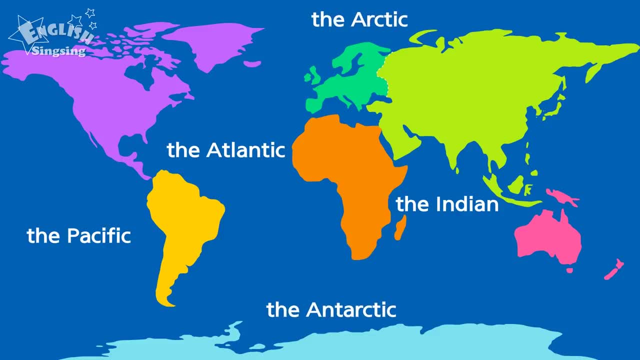 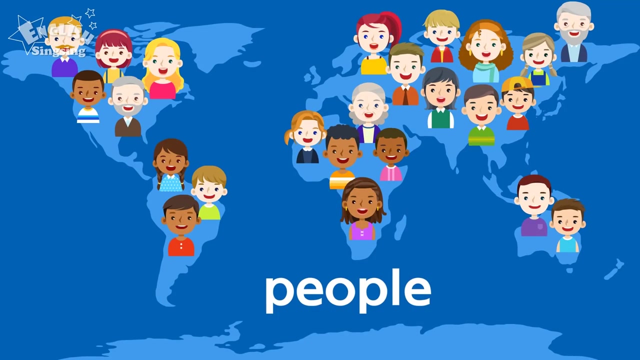 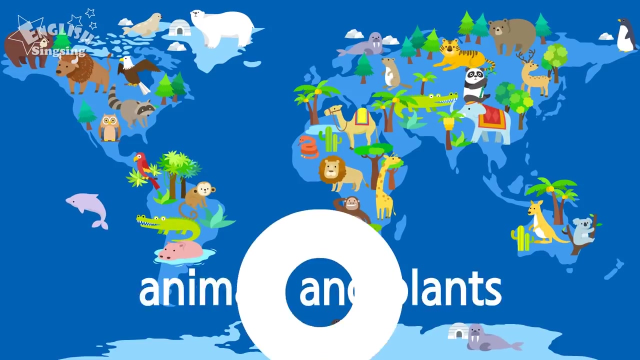 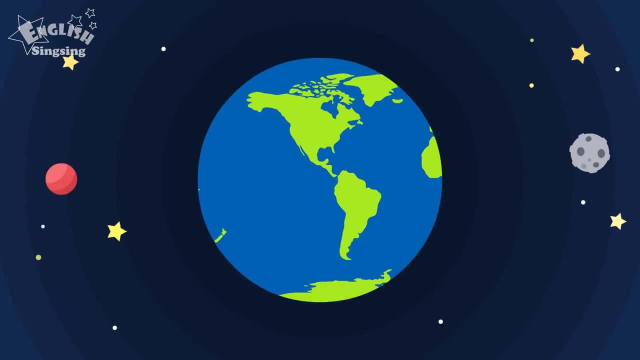 the Indian, the Antarctic and the Arctic Countries: There are about two hundred countries on the Earth. Countries, People: There are over seven billion people on the Earth. People, Animals and Plants: There are various animals and plants on the Earth. Animals and Plants. Earth: This is our planet Earth. 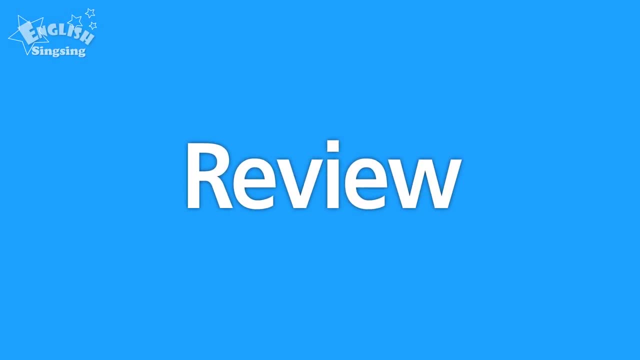 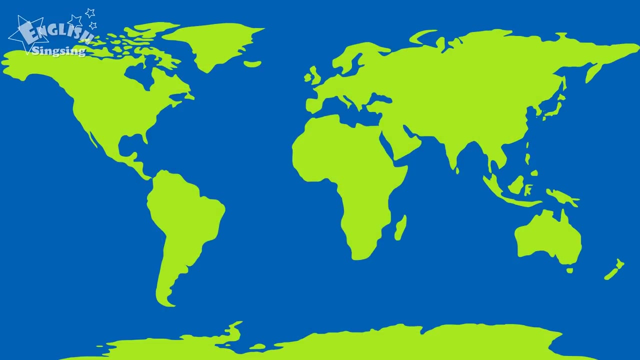 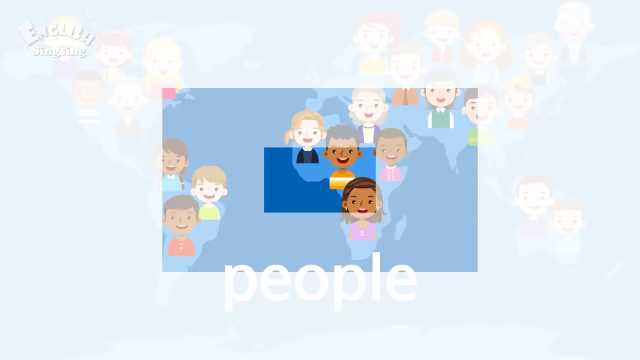 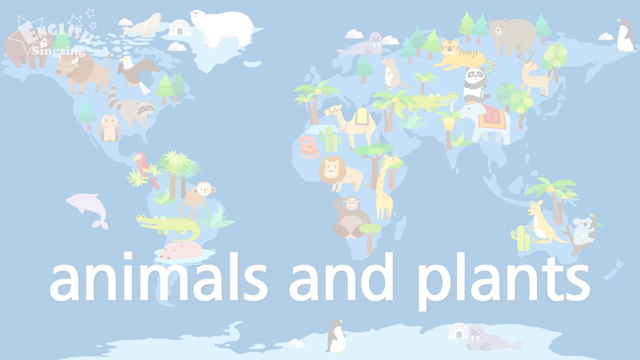 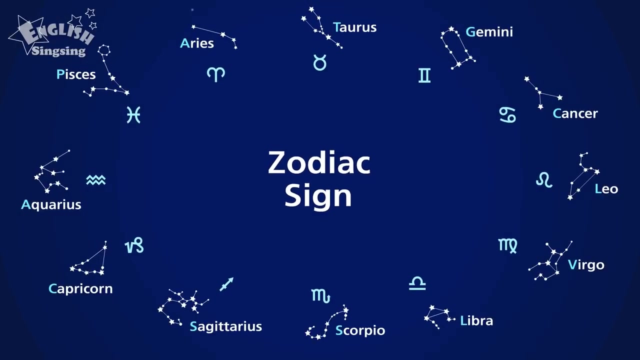 Earth Review. Earth Continents: Asia, Europe, North America, South America, Africa, Oceania, Antarctica, Oceans, Earth, Earth, Earth Earth- Pacific, Pacific, Atlantic, Indian, Indian, Antarctic, icut Countries, People, Animals and plants. Zodiac sign: Earth. Aquarius, Pisces, Aries, Taurus, Gemini, Cancer, Leo, Virgo, Libra, Scorpio, Sagittarius, Capricorn. Zodiac sign. 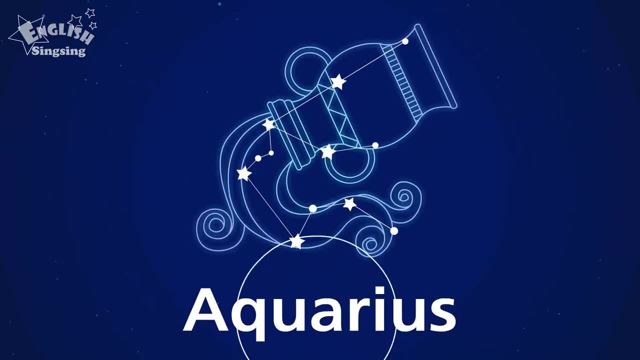 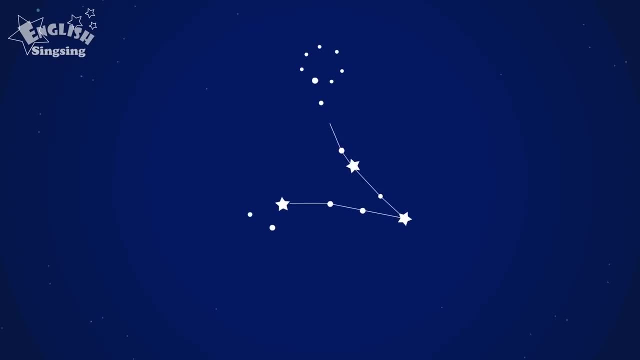 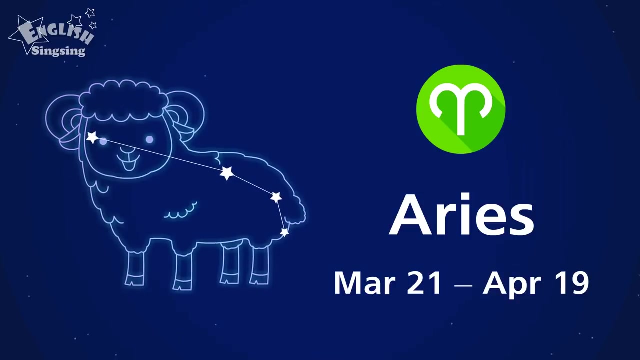 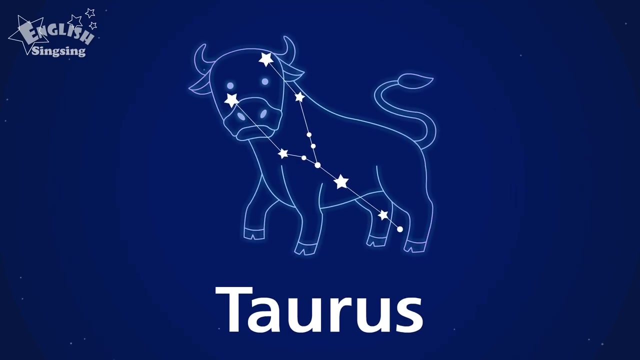 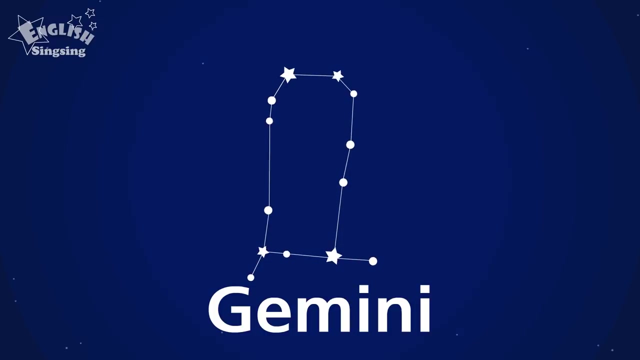 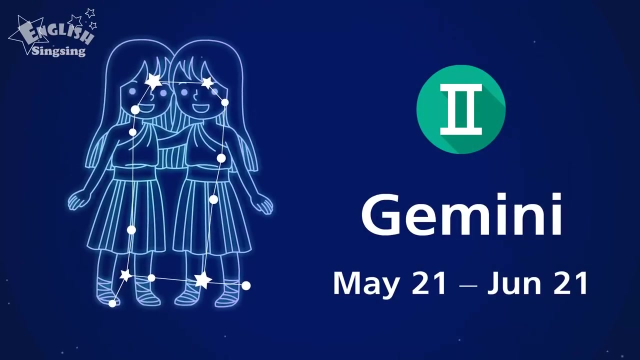 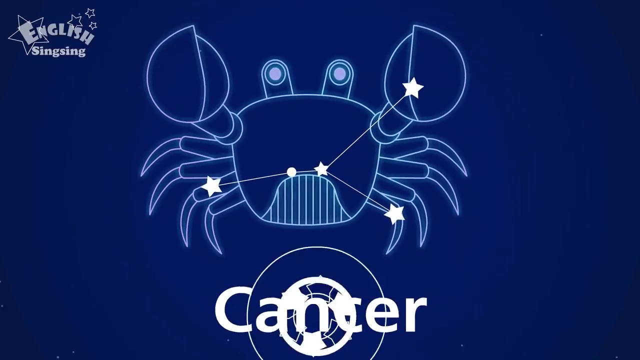 Aquarius, Aquarius, Aquarius, Pisces, Pisces, Pisces, Aries, Aries, Aries, Taurus, Taurus, Taurus, Taurus, Gemini, Gemini, Gemini, Cancer, Cancer, Cancer. 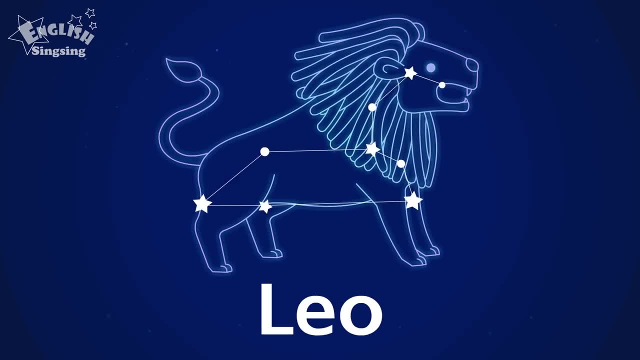 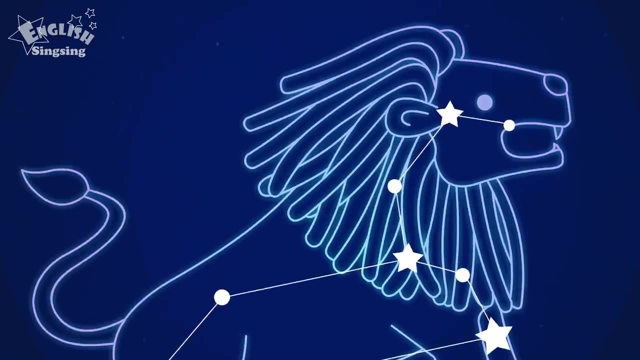 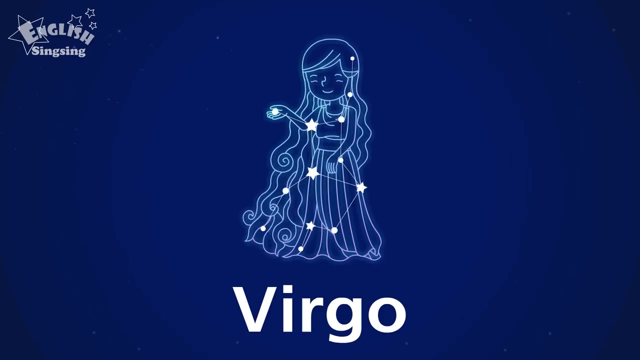 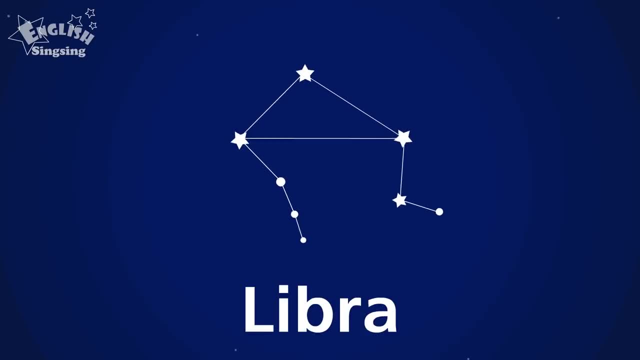 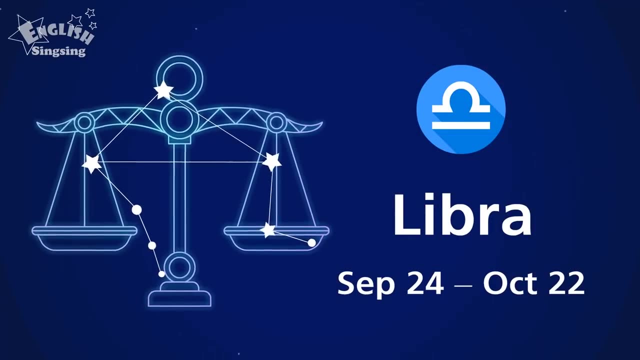 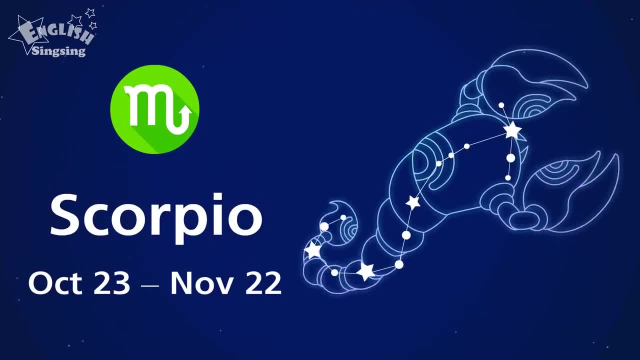 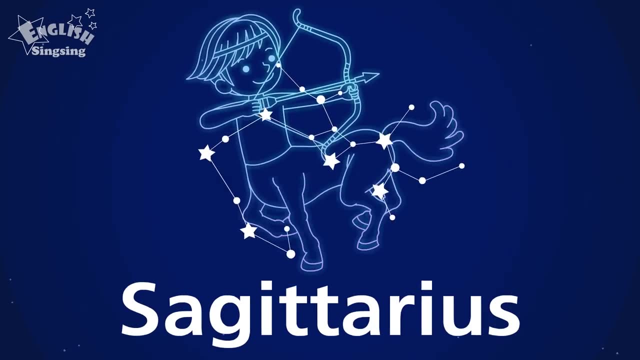 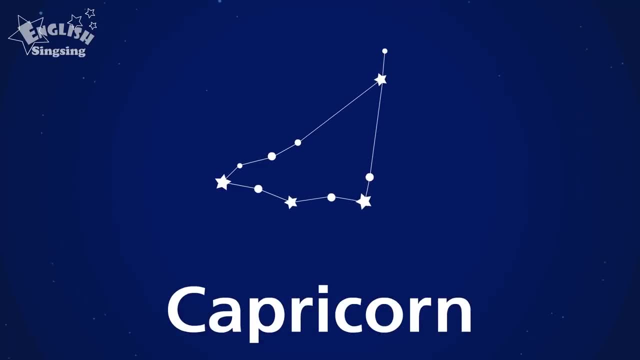 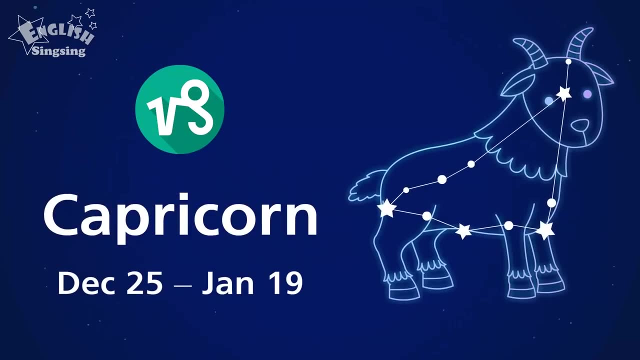 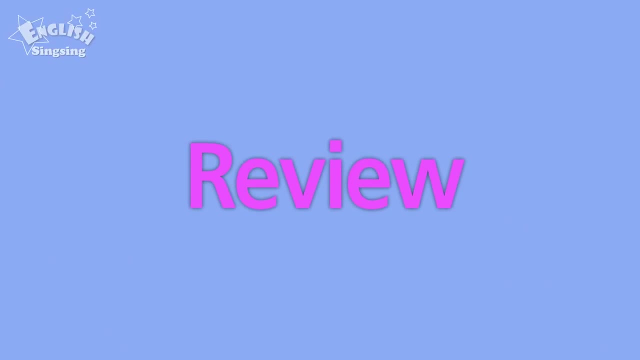 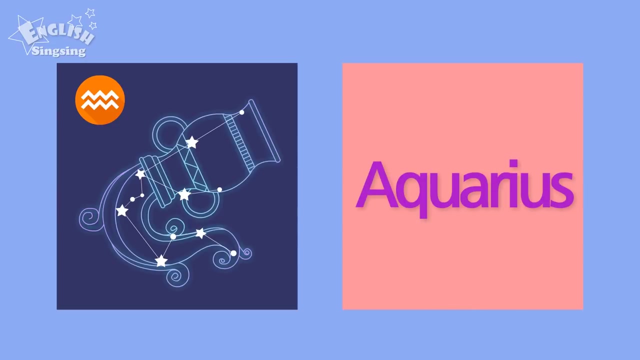 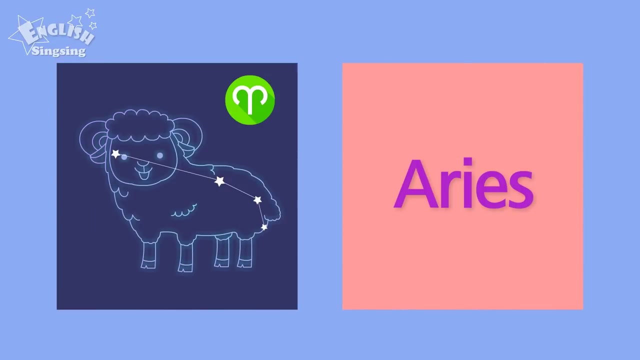 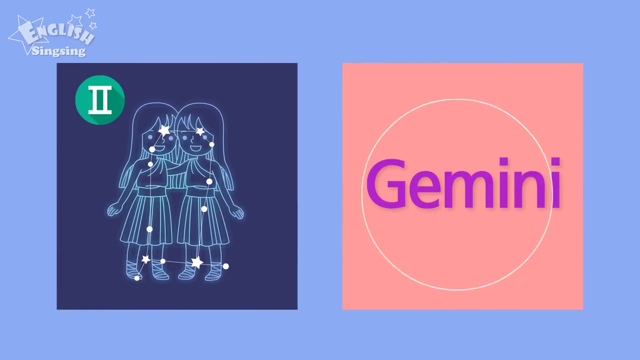 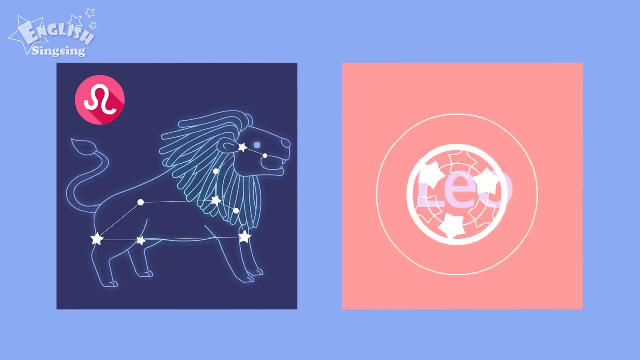 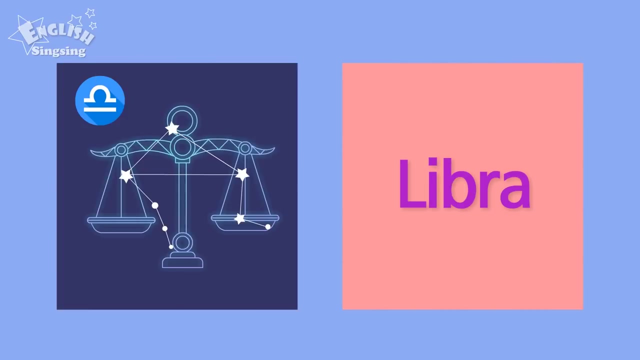 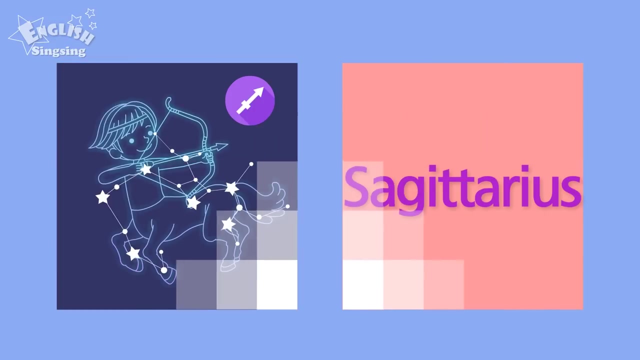 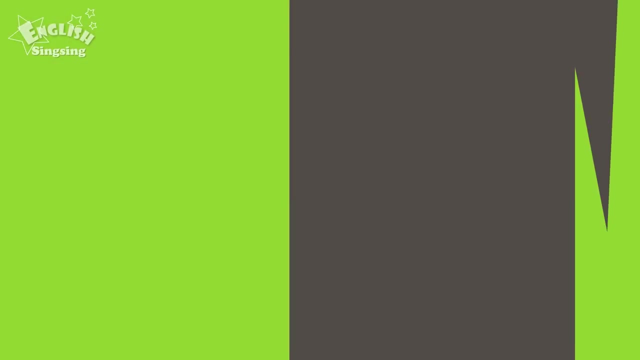 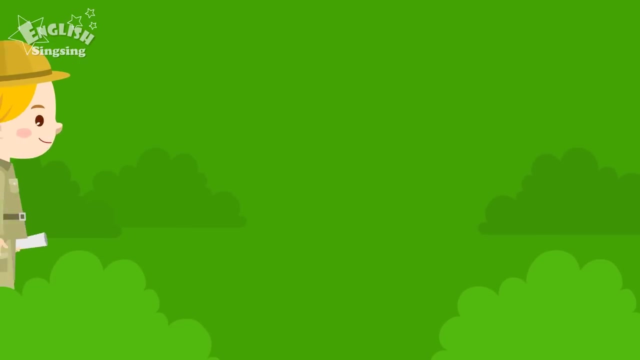 Virgo- Virgo- Virgo- Virgo- Virgo- Capricorn Zodiac Sign. Review Zodiac Sign: Aquarius, Pisces, Aries, Taurus, Gemini, Cancer, Leo, Virgo, Libra, Scorpio, Sagittarius- Capricorn Map. Hmm, let's see. 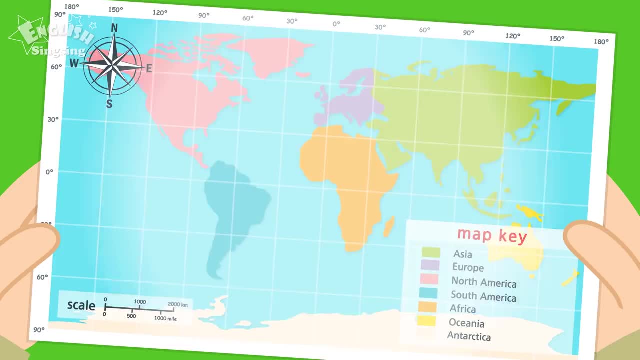 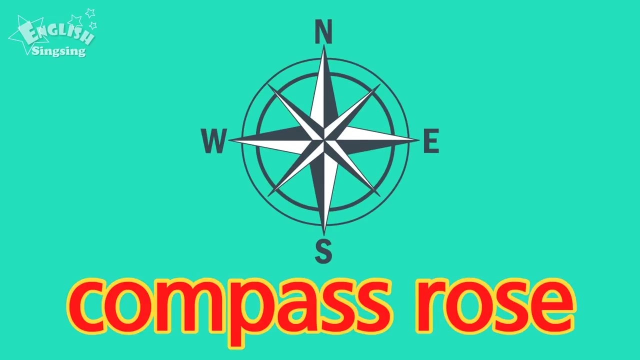 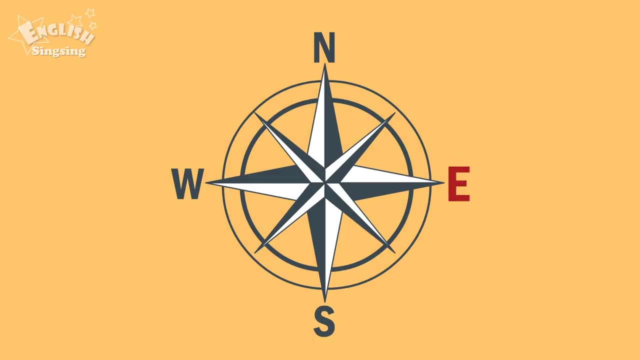 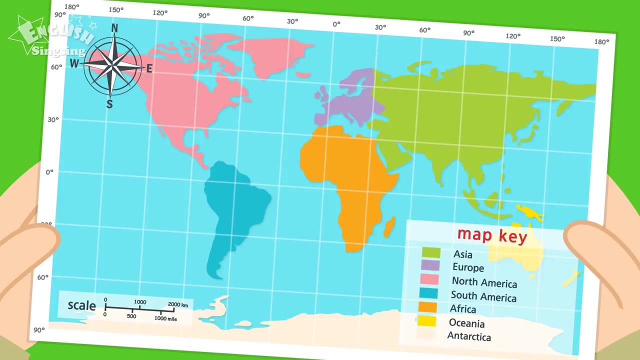 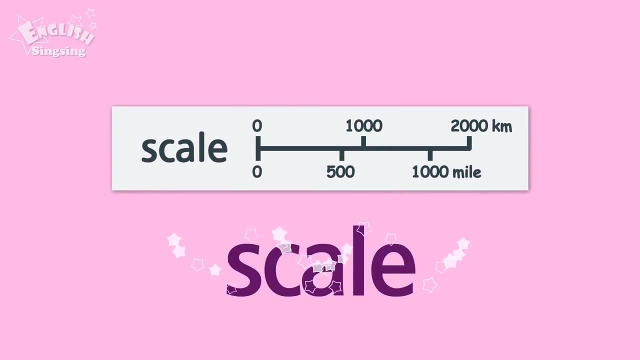 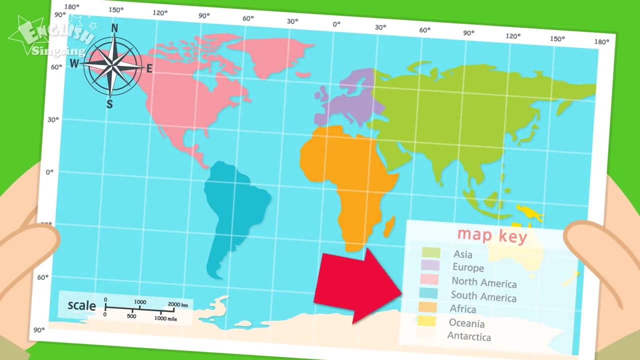 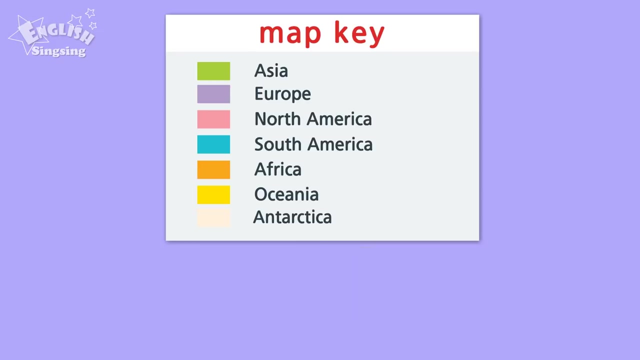 Wow, How to use a map. Map, It's a map. What's this Compass Rose? North, South, East, West- It's a compass rose. Ah, what about this Scale? It's a scale. What about this Map key? Map key, It's a map key.